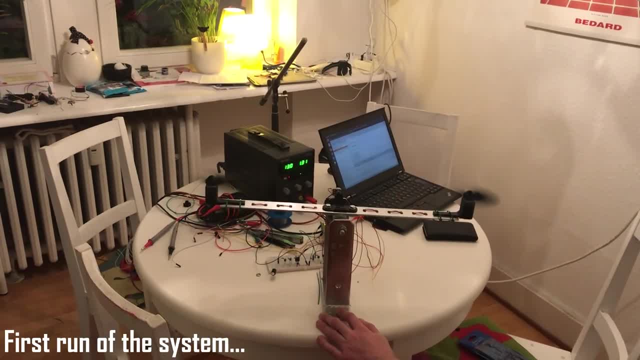 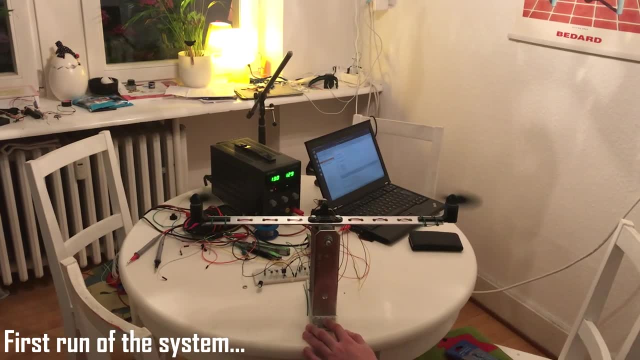 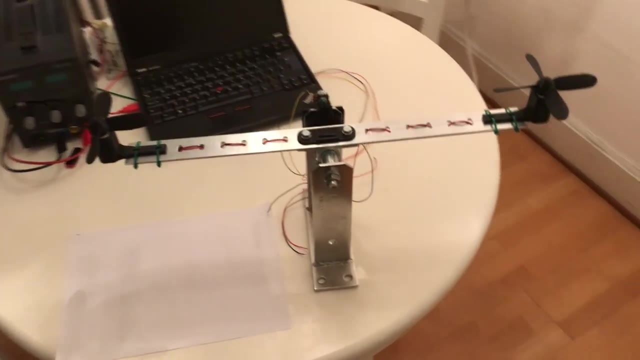 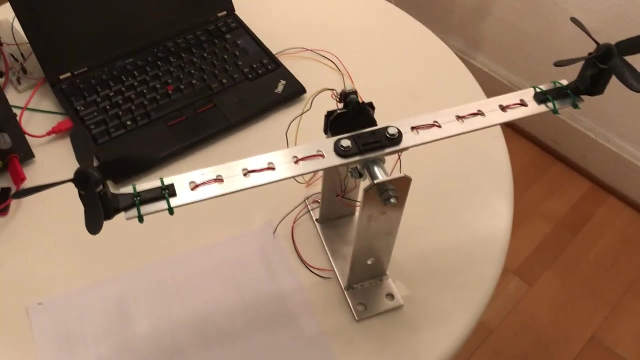 So this is the system we'll be looking at for the control system design videos. This is the balanced aero pendulum and this is what I've been making for the past one to two weeks. You can see here this is a kind of a stainless steel fixture. then I've put this rod and pivot mechanism up here. so 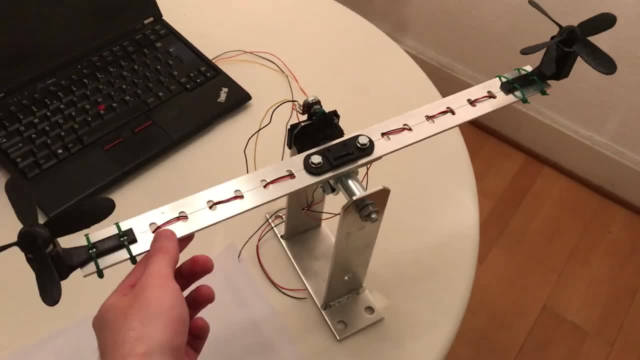 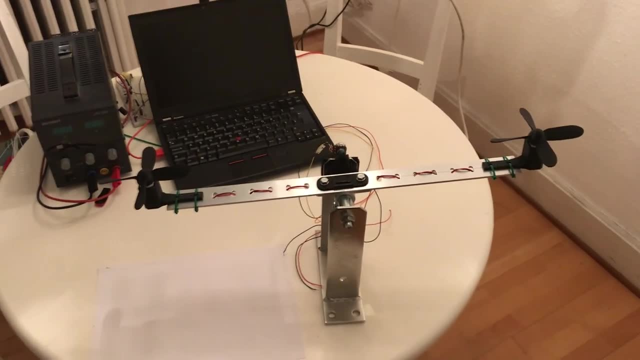 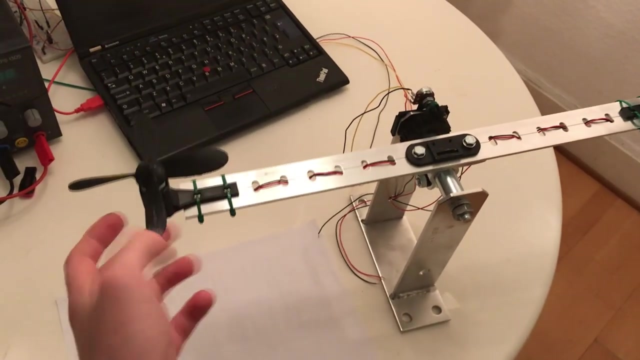 it's basically just an axle with a hollow steel shaft around it, so it can rotate about that point. At either end we have the DC brushed motors and propellers. I chose brushed motors because they're easier to drive. These mounts are 3d printed and the propellers are 3d printed on either end. So 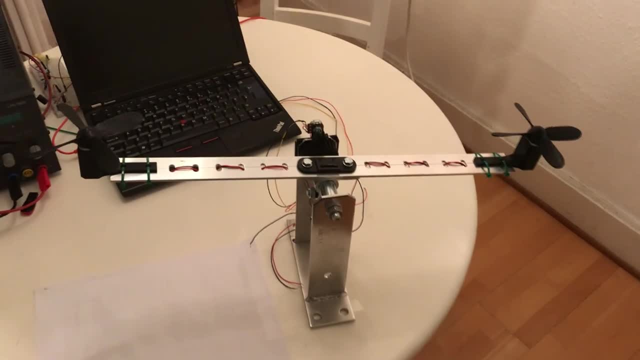 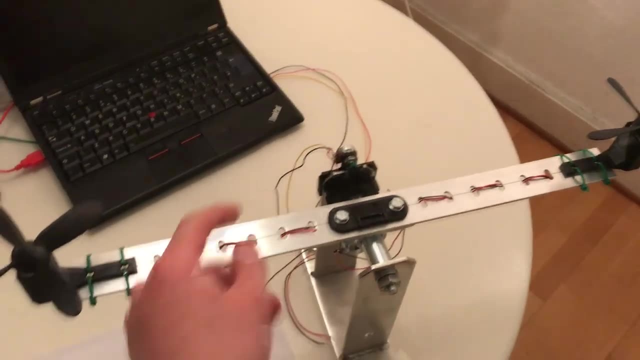 yes, so these are going to be our main actuators of these propellers and you can see if we rotate freely about the pivot with relatively little friction. the way we're sensing the angle is via this potentiometer and this little assembly over here. Now it's a bit hard to see in the light, but 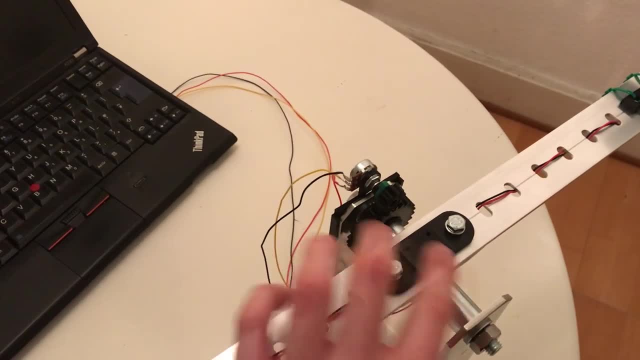 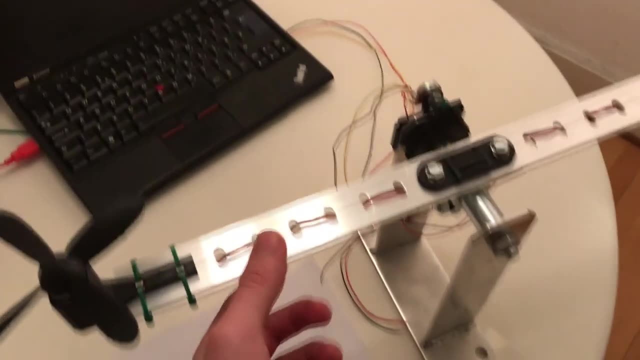 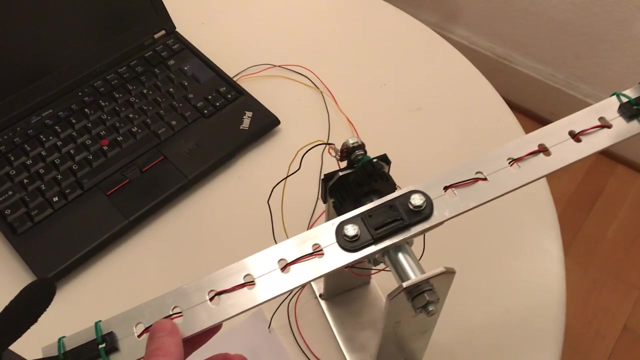 these are actually two gears, so one large gear attached to the pivot and then one smaller gear which is attached to the shaft of the potentiometer. so that way, when the larger gear rotates, the smaller gear rotates and that in turn rotates the shaft of the potentiometer. and we can just read: 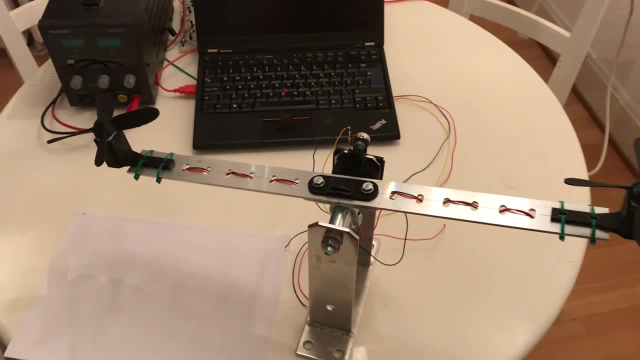 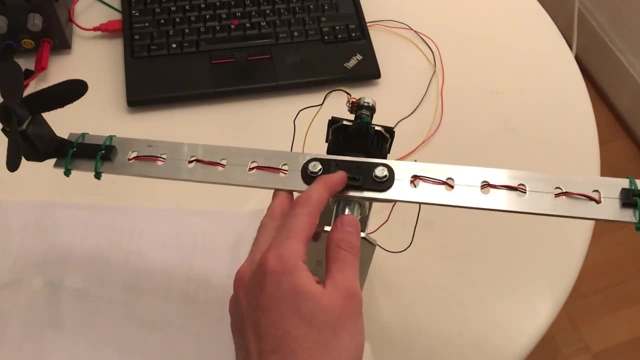 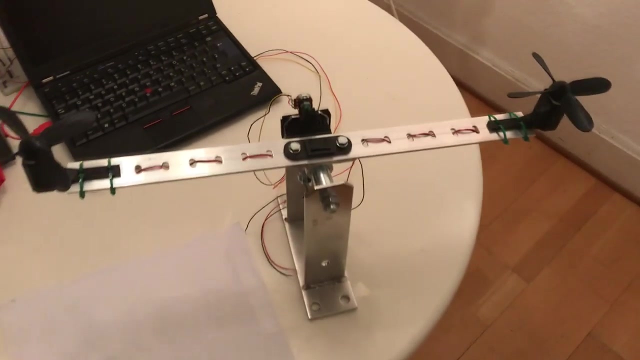 off an applied voltage. So that seems like a fairly simple solution to figuring out what angle this rod is currently at. You can see here I had actually 3d printed a mount for a natural measurement unit, but that sensor turned out to be far too noisy and I think this is a. 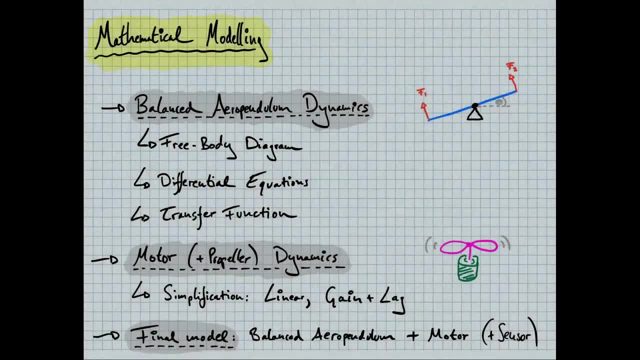 fairly elegant solution in place. Before we can design a control system, we need to have a mathematical model of the system dynamics we wish to control. In our case, the balanced arrow pendulum is the one we want to control, and the one we want to control is the one we want to control. 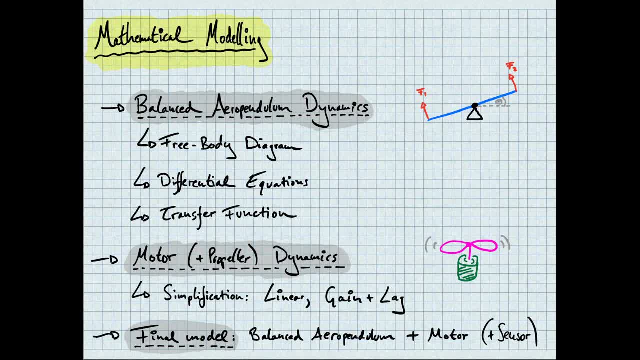 The balanced arrow pendulum turns out to be a fairly linear system with relatively simple equations of motion. To arrive at a system model useful for controller design, we start off by drawing a free body diagram defining system parameters such as masses, lengths, angles and so on, as well as showing all forces and moments acting on the system By using Newton's laws of 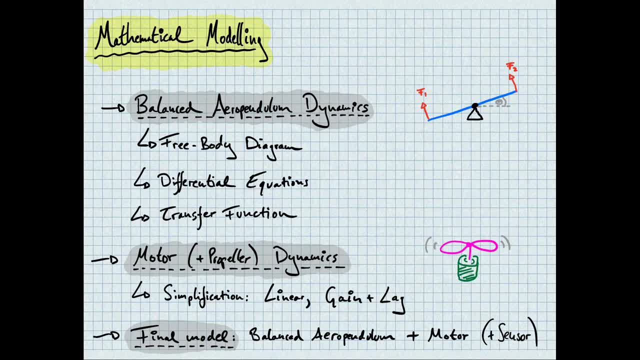 motion. we can sum these forces and moments to arrive at a governing differential equation. By applying the Laplace transform to this differential equation, we get a transfer function representation of the system. This is our basis for what we'll be using for control system design. However, this is not the whole story. To provide the forces that drive, 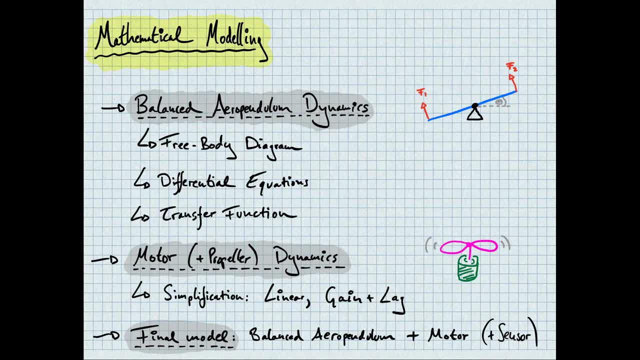 the system. we require actuators or, in our case, motors with propellers. The dynamics of these actuators also need to be taken into account. Finally, we'll combine the previously mentioned models with sensor and DAC approximations to arrive at the overall model of our system There. 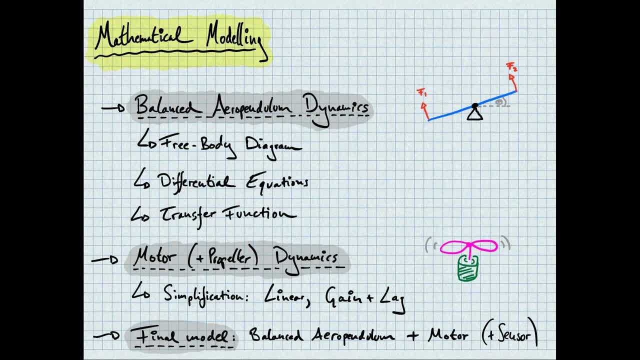 will be a fair amount of math to do to get the right model of our system. We'll also need to look at some other examples of maths in this video, so if you require any clarification, please leave a message in the comments. Without further ado, let's get started. 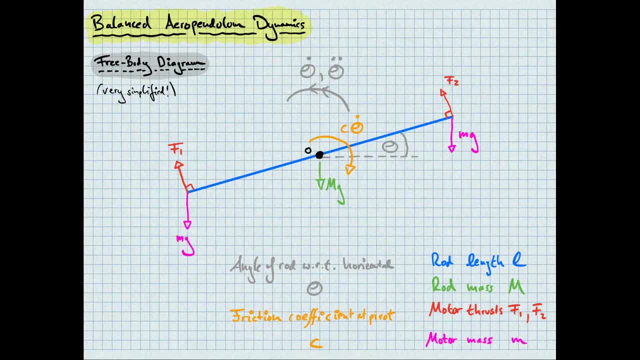 Shown here is the free body diagram of the balanced arrow pendulum. that is a rather simplified version. We assume that we have a thin rod of length L and of mass M rotating about a pivot at the rod center, which is this point O, The angle that the rod makes with a horizontal. 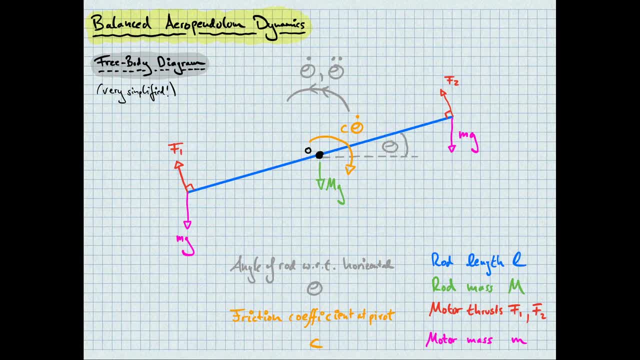 is denoted by theta. The angle that the rod makes with a horizontal is denoted by theta. We'll use this to define the average velocity. of course, At either end of the rod are motors with propellers, each of mass little m and each providing. 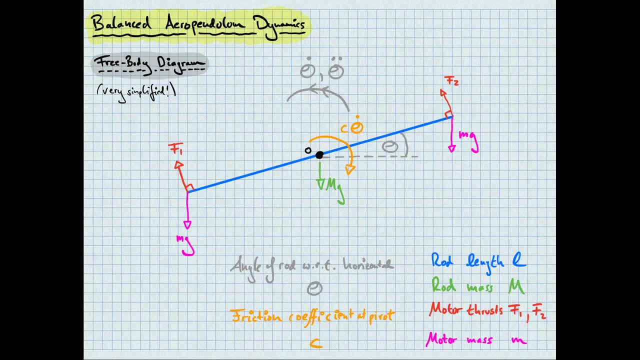 a thrust force: f1 and f2.. Finally, we will model the friction at the pivot via the friction coefficient c. The moment the friction generates is proportional to the rate of change of that angle and opposes the rotational motion of the rod. So if the rod is rotating counter-clockwise, the friction acts in the opposing direction. The moment the friction acts is proportional to the rate of change of the angle and the rotational motion of the rod. So if the rod is rotating counter-clockwise, the friction acts in the opposing direction. Thus the direction changes, which will result in a 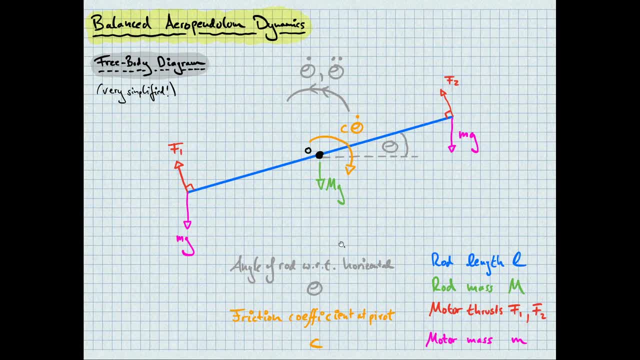 Thus, the larger value that C has, the more the system is damped. Now I have purposely left out finer details of this system. For instance, the masses of the motors will most likely not be identical, The rod is not thin, the friction coefficient is non-linear, and so on and so forth. 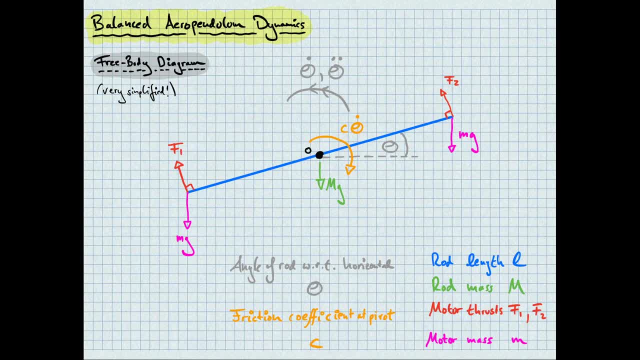 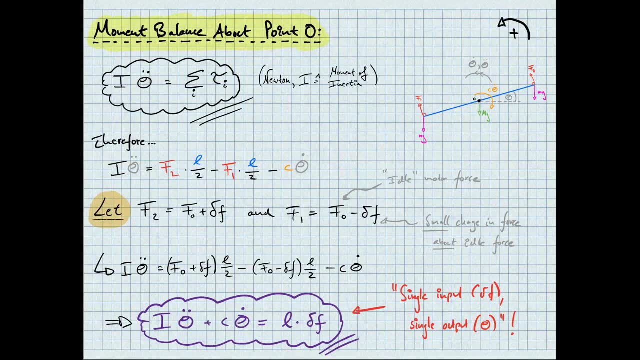 As is typically the case with control system design, we aim to design a controller that can cope with all expected parameter variations in the system. We now need to sum the moments of the free body diagram. The sum of moments, or torques rather, is equal to the angular acceleration. 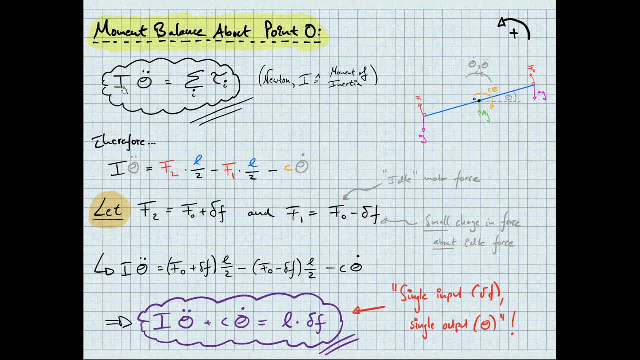 multiplied by the moment of inertia big I of the system- And this is from Newton's second law- The moment of inertia I is an object's resistance to rotational acceleration. This is analog to the mass in the case of linear acceleration. 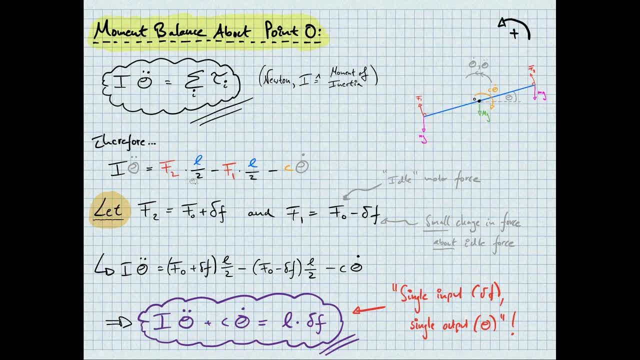 and we'll see how to calculate I later Now. the moment balance therefore becomes: by using this equation and then summing the torques this equation over here, And we get that by doing simple moment balance, we get the moment balance of the free body diagram. 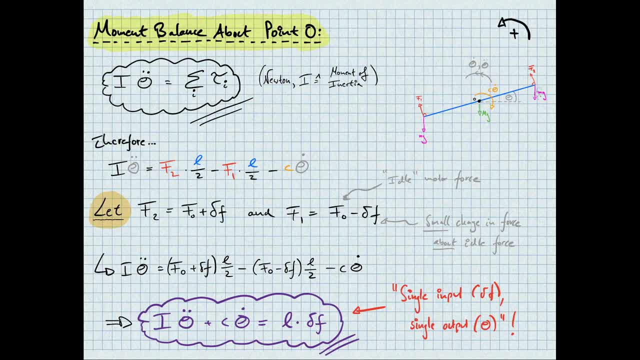 Now we have two motors each exerting a force- F1 and F2 respectively. but we can make our lives a lot easier by letting each motor run at the same idle force. so F0, so it's running at 50% duty cycle. 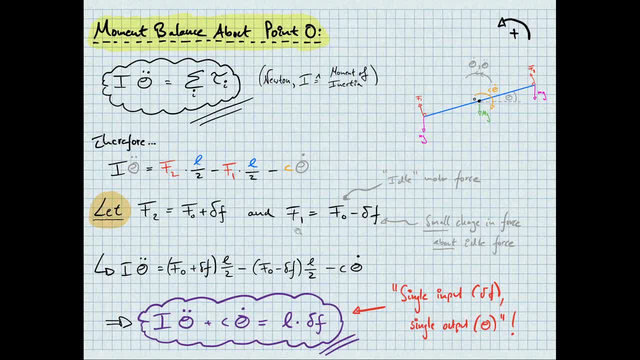 and then we have a plus minus perturbation- let's call it delta F- around that idle force. Now, instead of controlling two forces- F1 and F2, we simply control one force, Delta F. Now note the plus and minus sign difference. 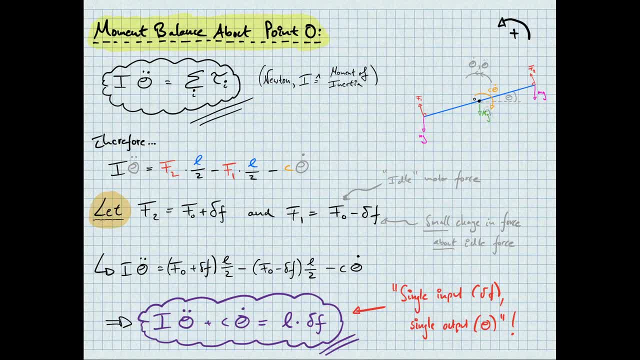 This is because F2, shown over here, tends to increase theta, whereas F1 tends to decrease theta. Substituting these new force expressions into the original equation over here yields the final single input, single output differential equation down here. Now this is great because we've substantially simplified the system into a single input, single output one. 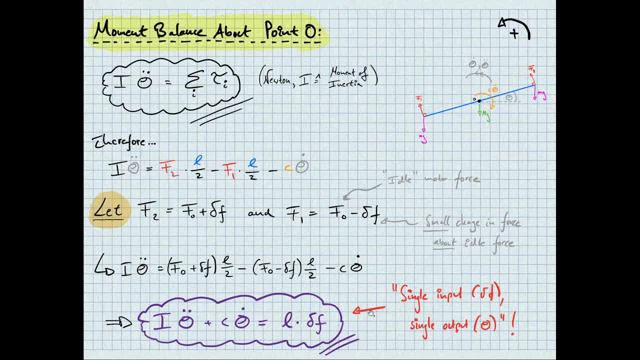 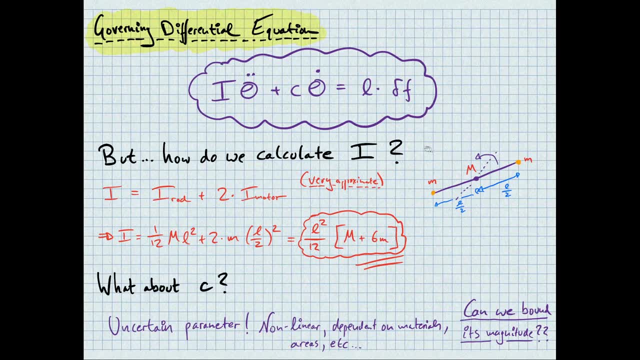 but also it is linear, which makes our lives a lot easier for controller design later on, With the differential equation in place, we may begin to wonder how we calculate the parameters of the system. so, for example, I or C. Let's have a brief look now, but I will go into greater detail in the next video. 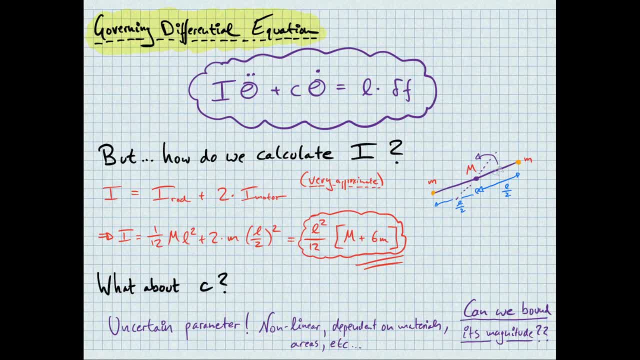 Now we can approximate the moment of inertia by assuming that the rod is thin and has two point masses, that is being the motor and propellers at each end. Now, using standard results, we arrive at a simple expression for the moment of inertia: 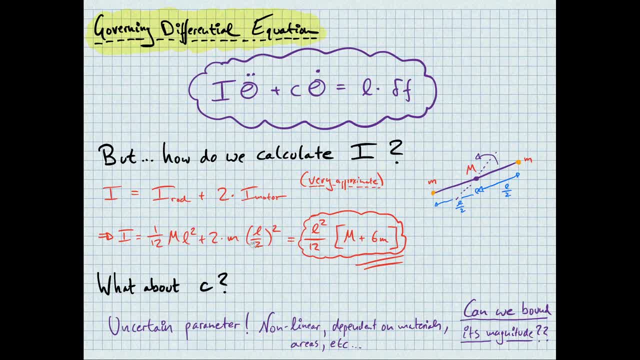 So we take the moment of inertia of the rod rotating about the centre, plus two times the moment of inertia of these point mass motors and we arrive at this expression. Now, remember, this is very approximate and I will calculate the moment of inertia in more detail in the next video. 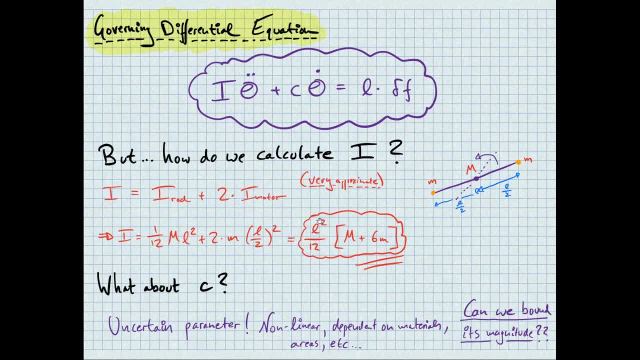 One thing to notice is that the magnitude of the moment of inertia is dependent on L squared, and also notice how it is dependent on the rod mass and also the motor mass. Now, more interestingly, what about C, the friction coefficient? This is a rather well, very uncertain parameter. 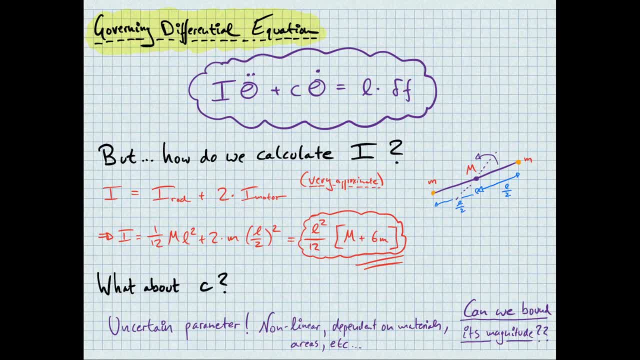 and we don't have direct ways of measuring it. It is non-linear, dependent on materials, areas, masses and so forth. But the question is: can we somehow bound its magnitude? So can we say it's between like zero and two. 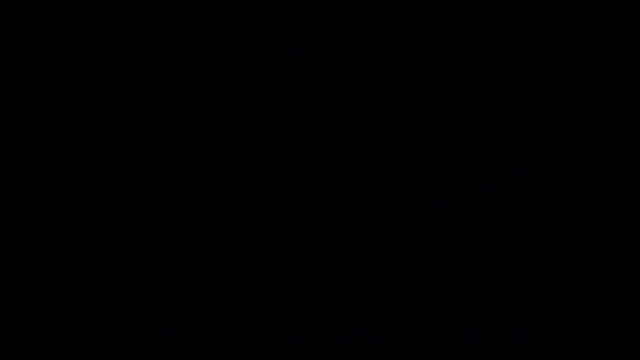 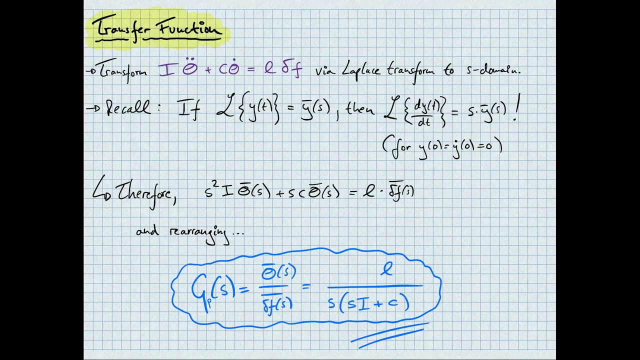 Now again, this is something we'll look at in detail in the next video. We now have all we need to convert the differential equation into a transfer function. This will be used for controller design later on. Recall that for zero initial conditions, the Laplace transform of a derivative. 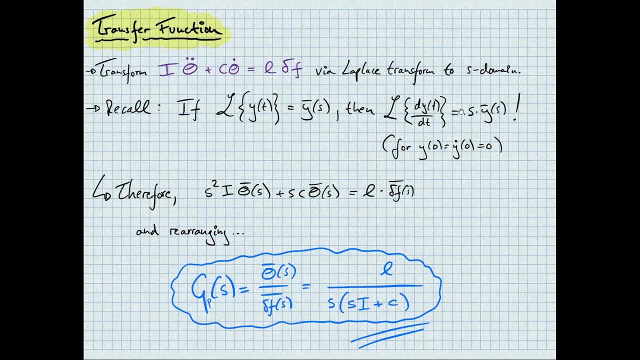 is simply the Laplace transformed variable multiplied by s. Therefore, combining this knowledge with the original differential equation, we arrive at this expression. Now, rearranging, we arrive at the transfer function for the balanced arrow pendulum. The input is the change in force delta f in Newton. 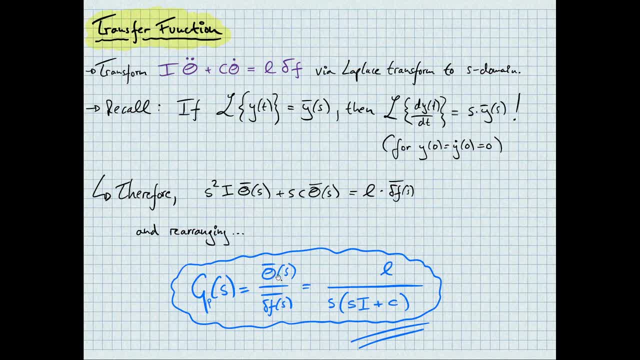 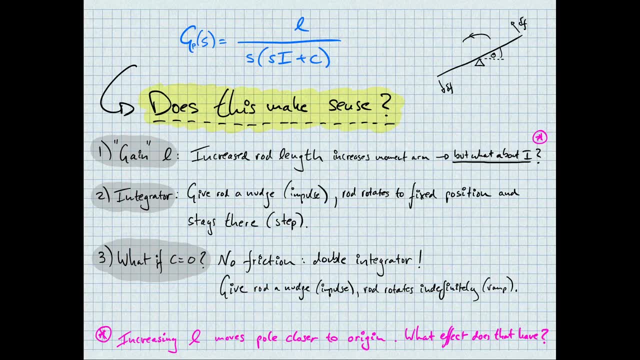 and the output is the angle of the rod with respect to the horizontal, and the units are in radians. Let's ask ourselves if this transfer function makes sense. I always find it useful to think if the transfer function intuitively represents the dynamics of the system. 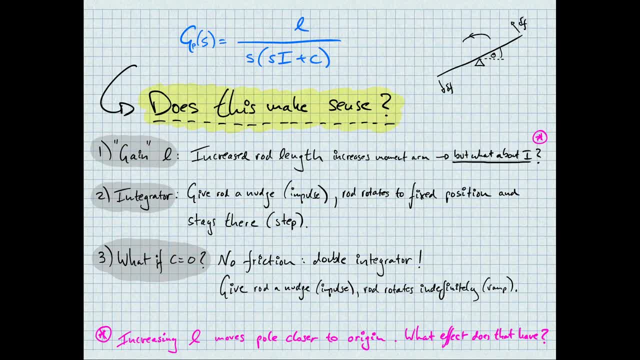 what we'd expect it to do, based purely on our everyday physical understanding of the world. Now, first of all, we have again L, which is the rod length. If we increase the rod length, the effectiveness or the moment arm of the motors is increased. However, recall that the moment of 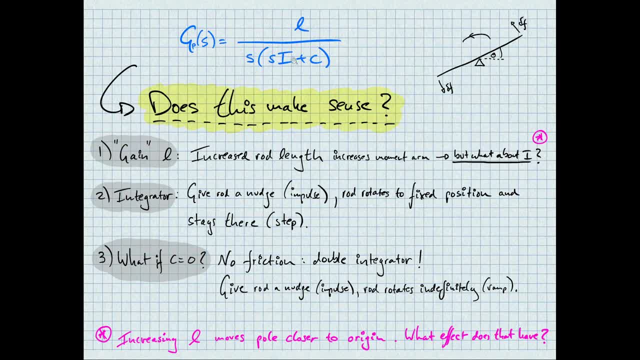 inertia actually increases with L squared, and that's in the denominator over here. Additionally, increasing L moves one of the poles closer to the origin. Secondly, the system has a pole of the origin, which is this 1 over S term over here. This is an integrator, So intuitively. 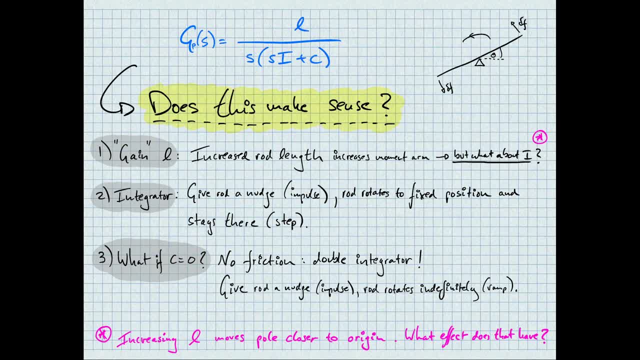 if we give the rod a nudge, an impulse input, the rod rotates to a fixed position and stays there, and that means that's a step output. Lastly, we can ask ourselves what happens if we change C? What happens if there's no friction? 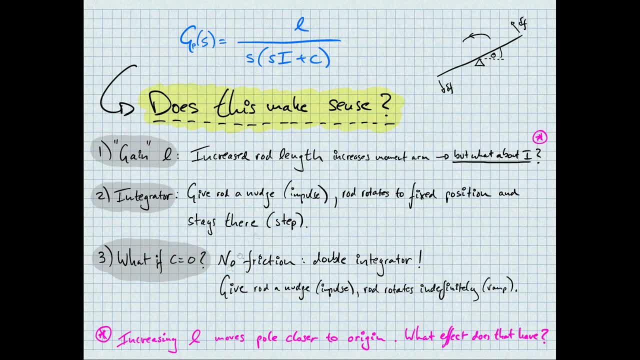 So if we change C, what happens? if there's no friction? That means C equals zero. Now this means that we have two poles of the origin. So for C equals zero, we have S squared in the denominator. That means we have a double. 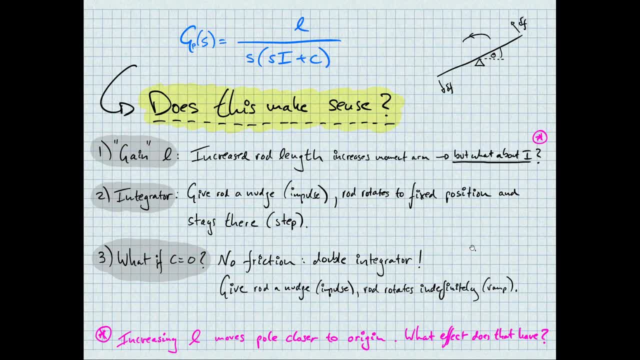 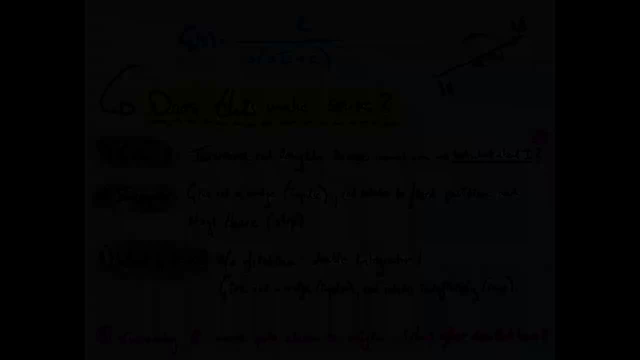 integrator. Now, if you give a rod a nudge, as in an impulse input, the rod will rotate indefinitely, and that is actually a ramp output. So what we'd expect from a double integrator- Motor and propeller modeling is a huge topic in its own right and something that would take a 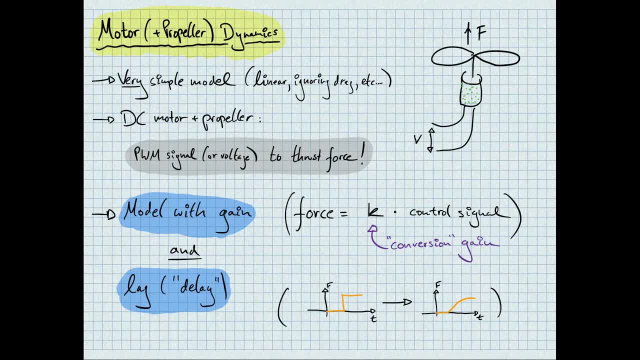 very long time to cover in any great detail. We therefore restrict our model to a rather simple one. We ignore non-linearities, drag friction and so forth. Ideally, we want a model or transfer function where we apply a voltage or PWM duty cycle and the output is: 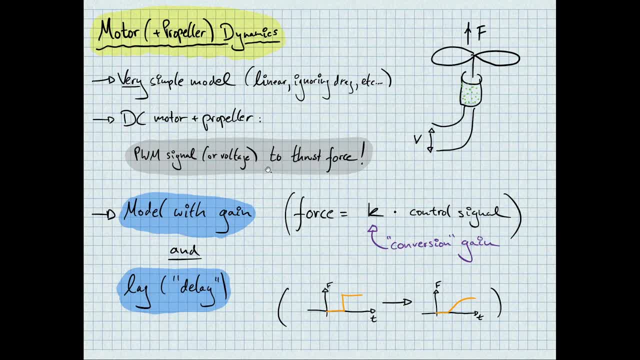 the resulting thrust force. We can do this by modeling this conversion from voltage to force via a gain which we'll call k. This gain is the linearization of the motor's transfer characteristic at a certain idle, RPM or operating point, so to speak. However, we also know that the 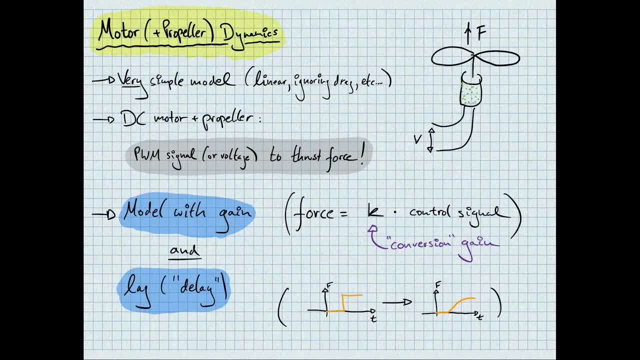 motor's speed, which is the speed of the motor, is less than the speed of the motor itself. This is why the speed, and therefore its thrust, cannot change instantaneously. We can model this effect via a lag or a delay term. This way, a step input results in an exponentially increasing output. 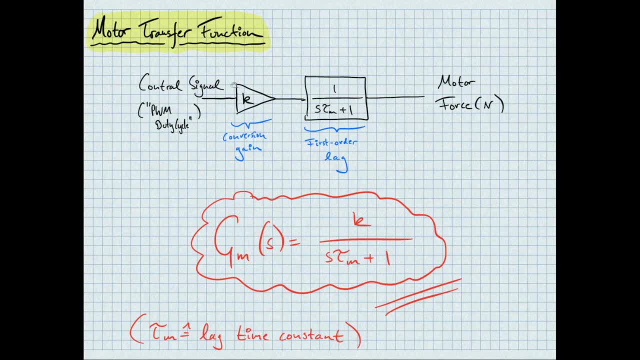 The motor transfer function is therefore simply the cascade of the conversion gain and the first-order lag. The first-order lag can also be seen as a low-pass filter where high-frequency components are attenuated. Tau m is the lag time constant If. 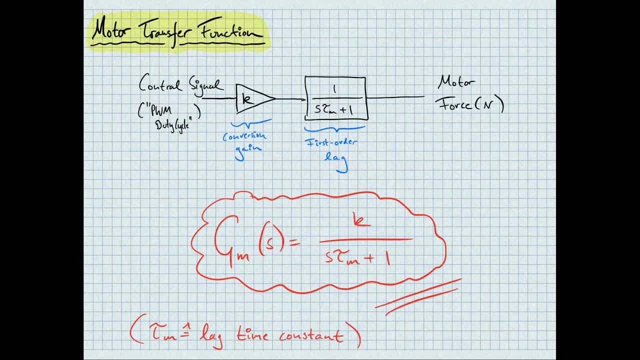 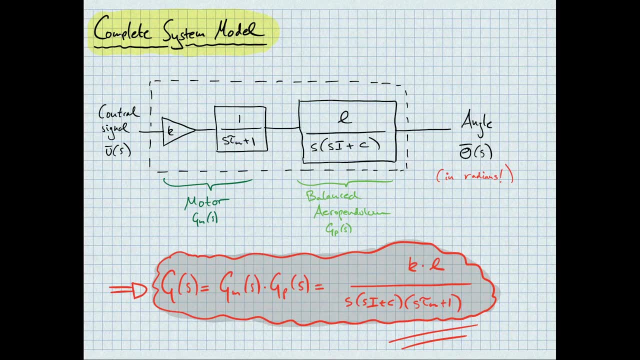 tau m is zero, the lag disappears. In other words, if tau m is large, there is a larger delay introduced into the system. The overall system model is essentially the cascade of the dynamics of the balanced aero-pendulum with the motor model we just derived, and this is then the overall 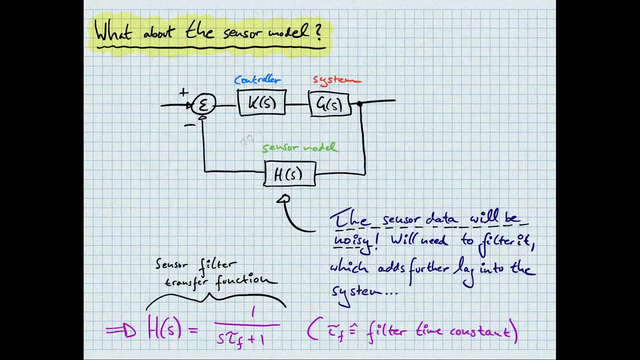 transfer function. But what about the sensor model, you might ask? In the real world, we'll be facing many non-idealities, for instance noisy sensors. We'll have to filter these noisy measurements, but this in turn will introduce additional lag or delay into the system. We will have to take this into account as too.